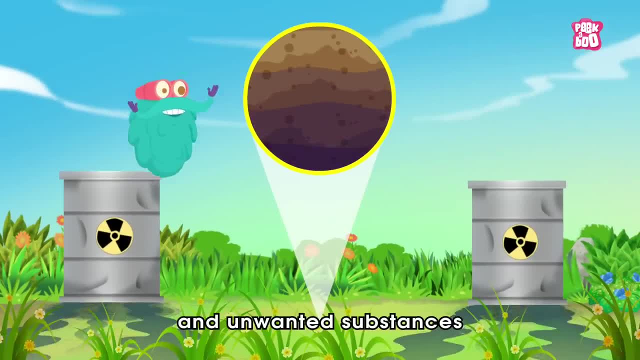 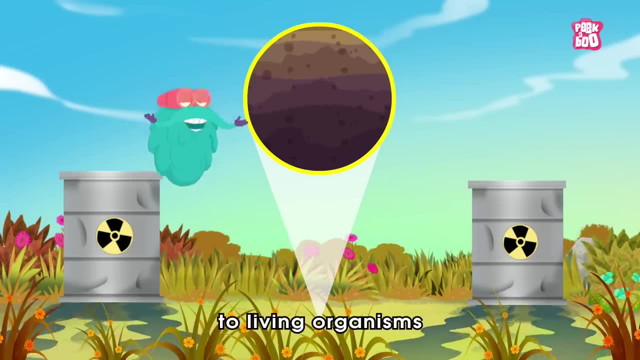 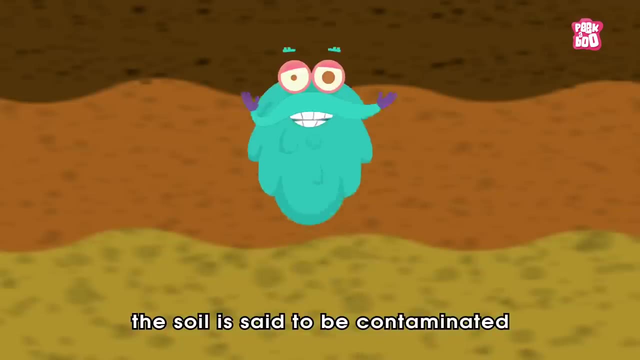 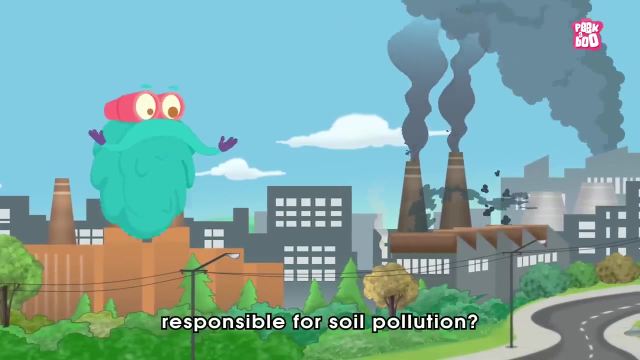 In other words, when the level of such toxic and unwanted substances in the soil increases enough to cause severe damage to living organisms such as plants, animals and humans. the soil is said to be contaminated or polluted, But what are the factors responsible for soil pollution? 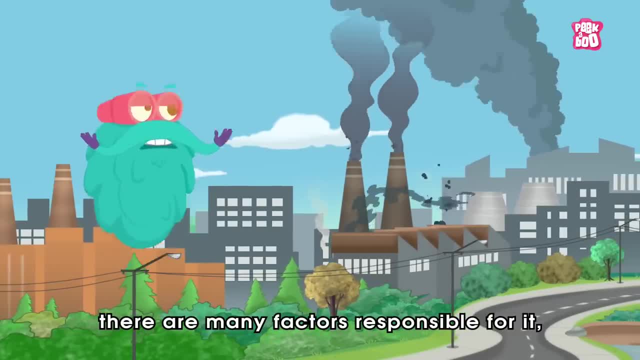 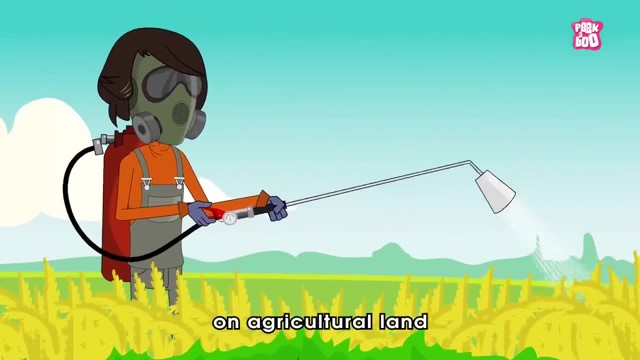 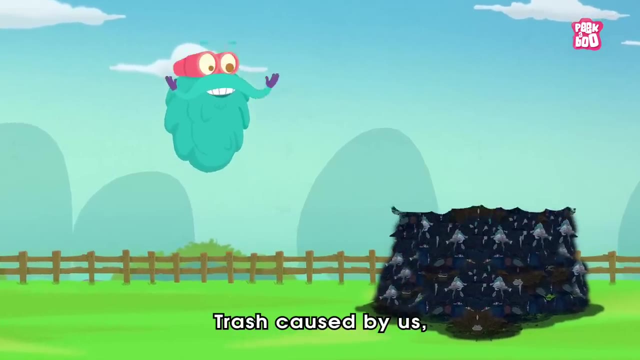 Well, there are many factors responsible for it, From the waste produced at giant factories to excessive use of pesticides on agricultural land, to the trash we throw away in our homes and school. Yes, dear friends, trash caused by us is one of many ways that soil gets polluted here on earth. 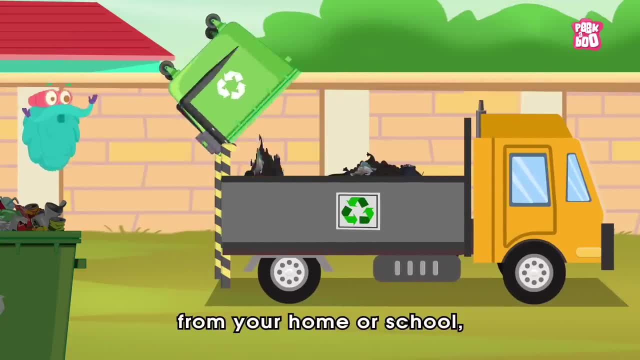 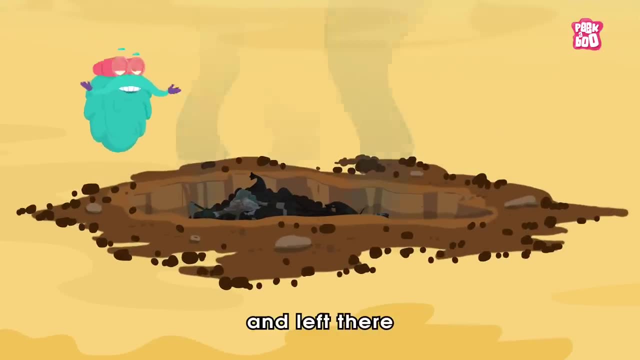 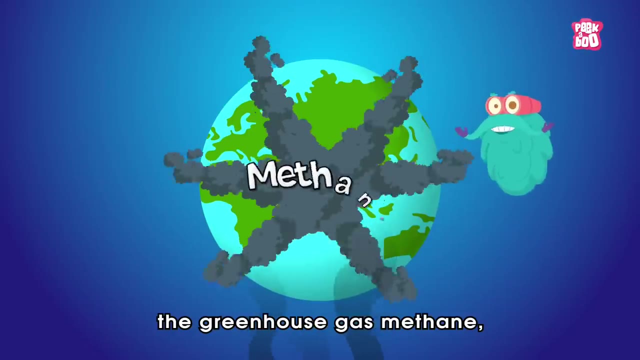 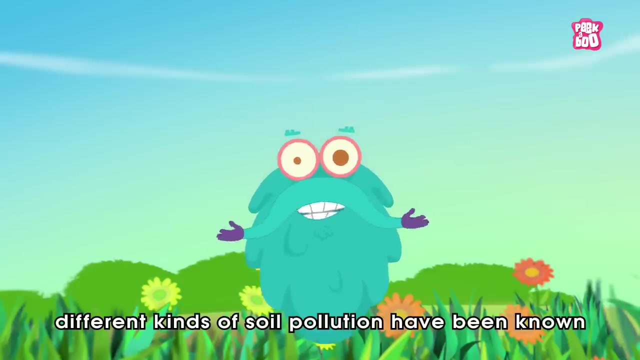 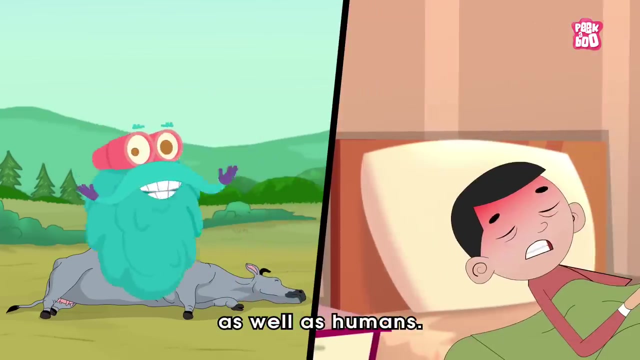 Once the garbage is picked up from your home or school, it is brought to a landfill, where it's buried in soil and left there to decompose or break down over time, which releases the greenhouse gas, methane, which may lead to global warming. Not only that, different kinds of soil pollution have been known to have adverse effects on the health of both animals as well as humans. 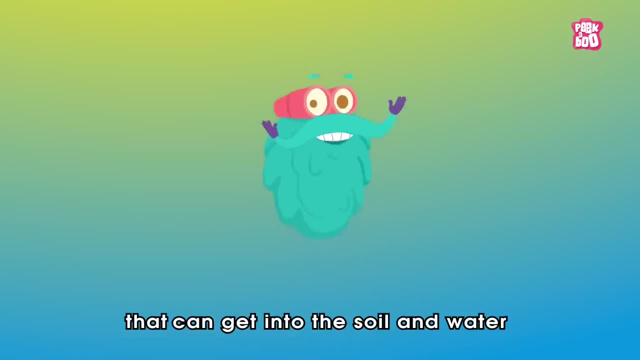 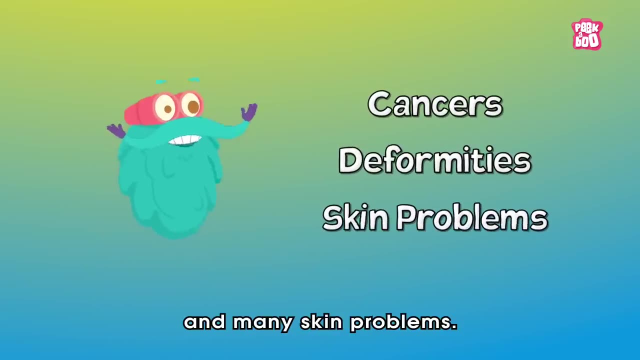 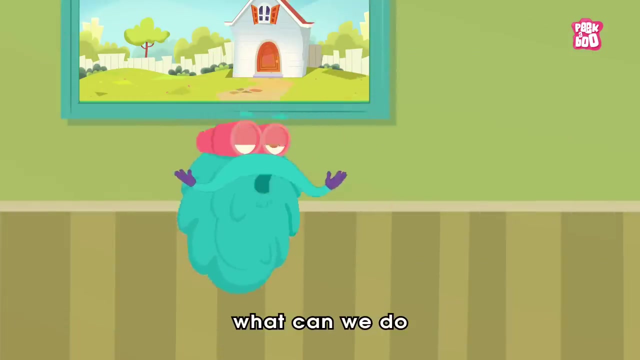 As the harmful chemicals that can get into the soil and water can cause cancers, deformities and many skin problems. So here comes the most crucial question: What can we do to prevent soil pollution? Well, as they say, if you want to change the world, start with the man in the mirror. 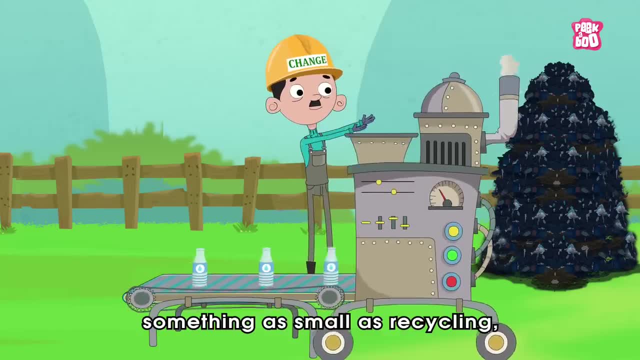 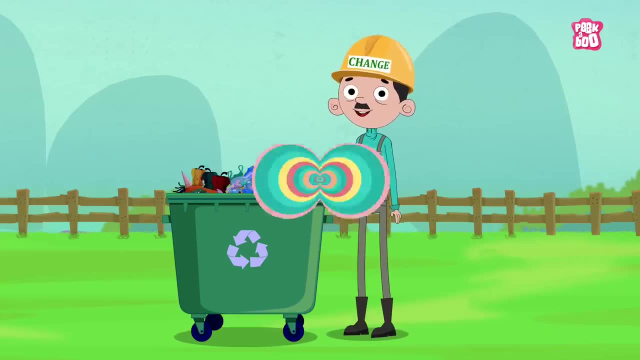 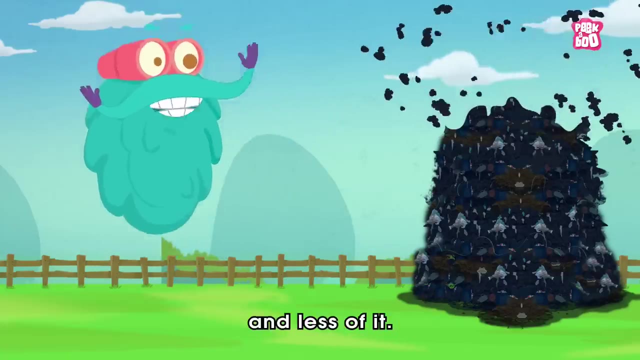 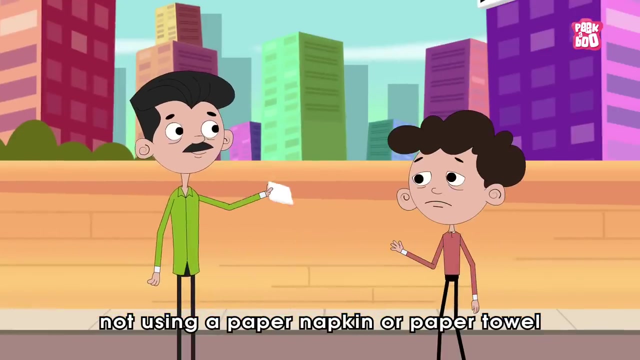 Yes, my friends, something as small as recycling, picking up trash from your surroundings, can make a huge difference, But the most important thing you can do to control waste is by producing less and less of it, And some ways to do so include not using a paper napkin or paper towel unless you absolutely need one.